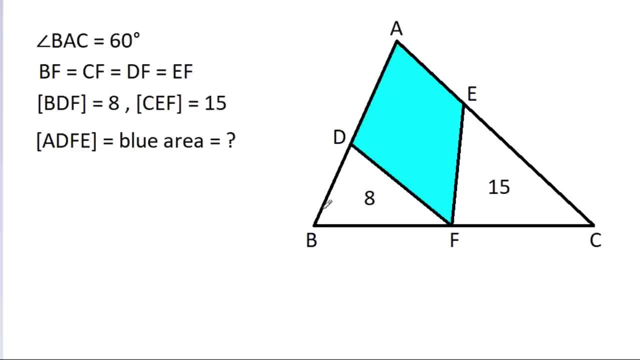 In this video we have given that angle: BAC it is 60 degree and BF it is equal to CF, it is equal to DF and it is equal to EF and area of BDF is 8, and area of CEF is 15,. 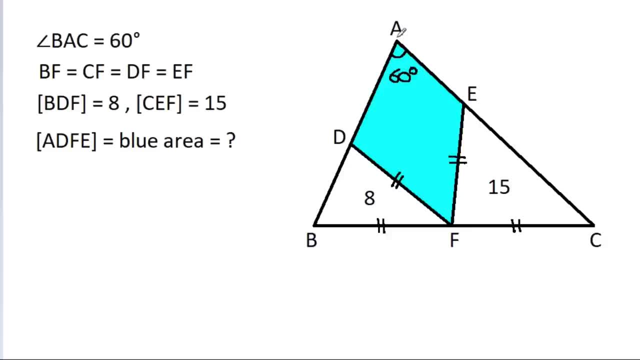 then we have to find area of ADFE. So in triangle A, B, C, suppose this angle is B and this angle is C, then 60 degree plus B plus C it will be equal to 180 degree. 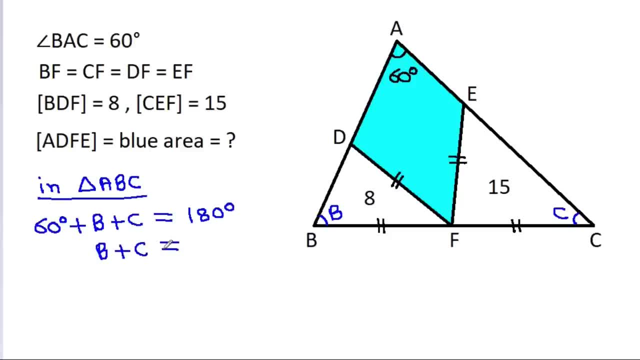 So B plus C it will be equal to 120 degree, And in any triangle- A, B, C- if AB is equal to AC, then these two angles will be equal, And here CF, it is equal to DF, so this angle will be also B. 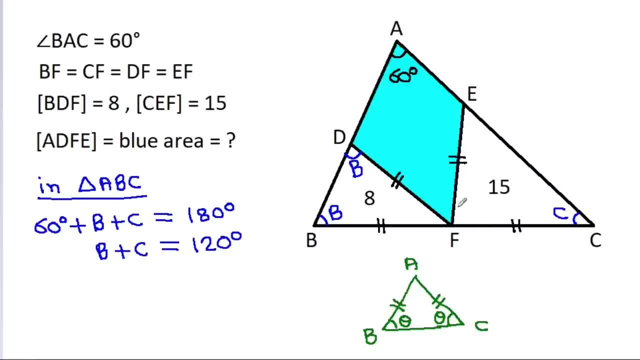 and CF, it is equal to EF. so this angle will be also C. And suppose this angle is P and this angle is Q, then in triangle BDF, B plus B plus P, it will be equal to 180 degree. 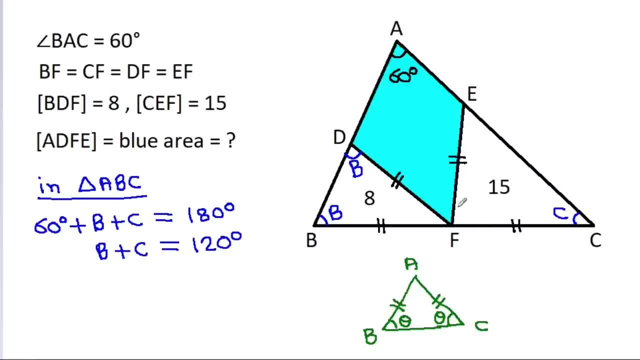 and CF, it is equal to EF. so this angle will be also C. And suppose this angle is P and this angle is Q, then in triangle BDF, B plus B plus P, it will be equal to 180 degree. 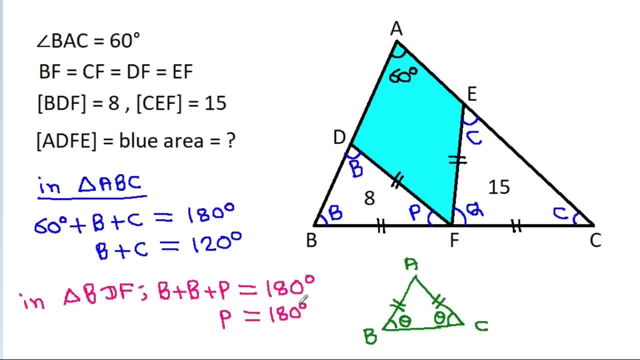 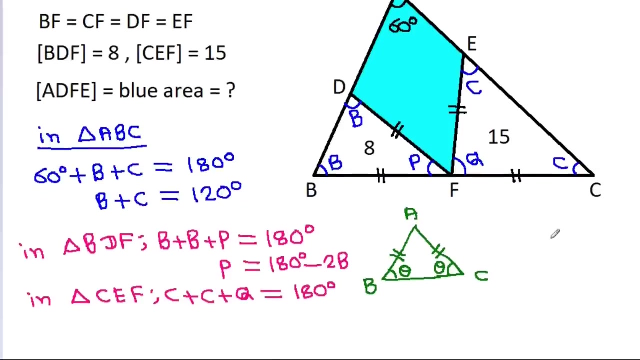 So P will be equal to 180 degree minus 2B And in triangle C, EF, C plus C plus Q, it will be equal to 180 degree. So Q will be equal to 180 degree minus 2C. 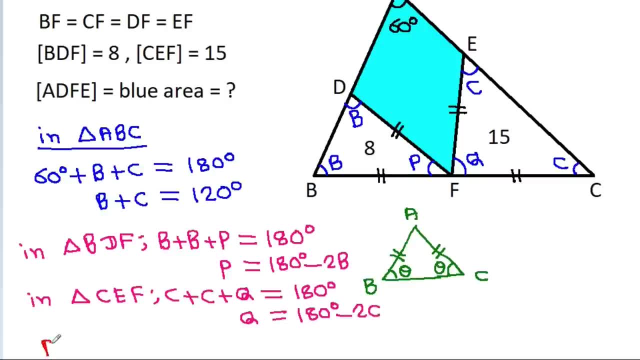 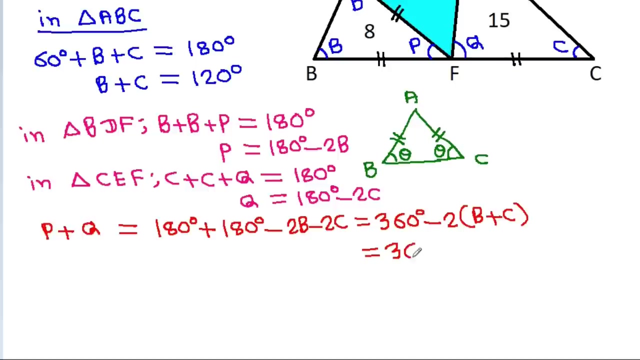 So P plus Q it will be equal to 180 degree plus 180 degree minus 2B minus 2C, And it is 360 degree minus 2 times B plus C. And it is 360 degree minus 2 times b plus c is 120 degree. 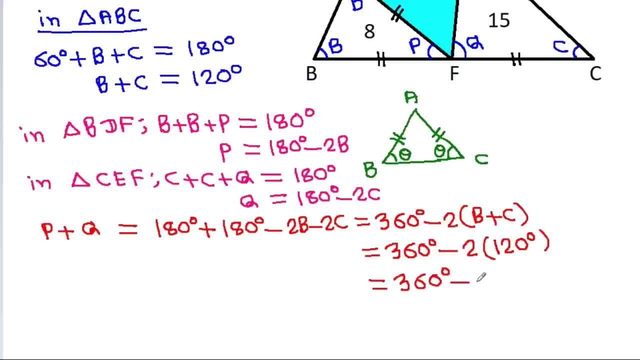 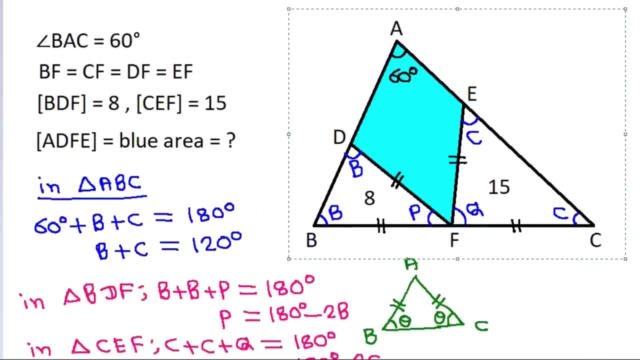 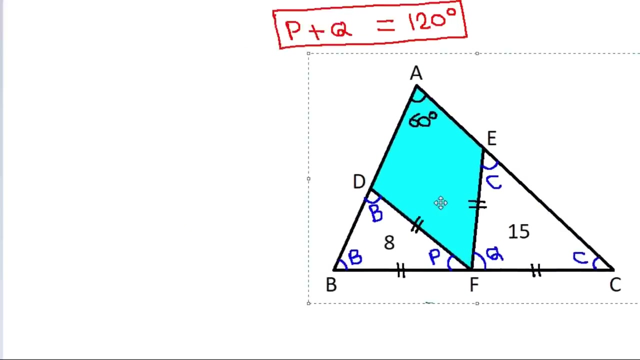 And it is 360 degree minus 240 degree, that will be equal to 120 degree. So p plus q, it is 120 degree. And now p plus angle df, e plus q, it will be equal to 180 degree, And p plus q is 120 degree. 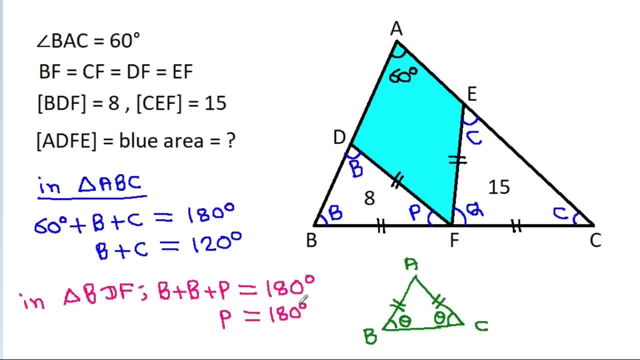 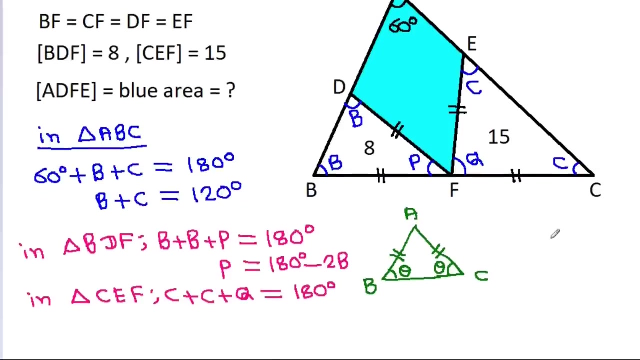 So P will be equal to 180 degree minus 2B And in triangle C, EF, C plus C plus Q, it will be equal to 180 degree. So Q will be equal to 180 degree minus 2C. 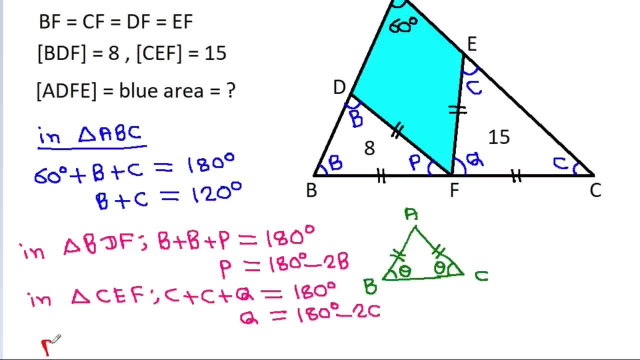 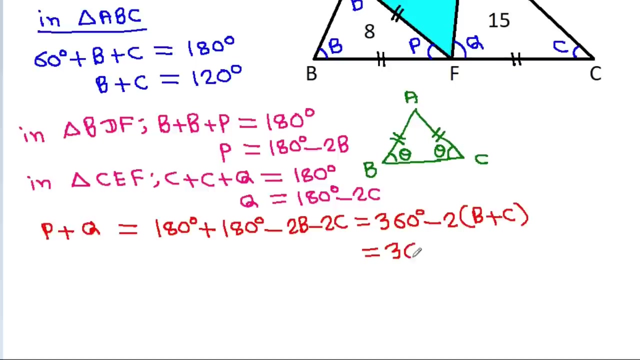 So P plus Q, it will be equal to 180 degree plus 180 degree minus 2B minus 2C, And it is 360 degree minus 2 times B plus C, And it is 360 degree minus 2 times B plus C. 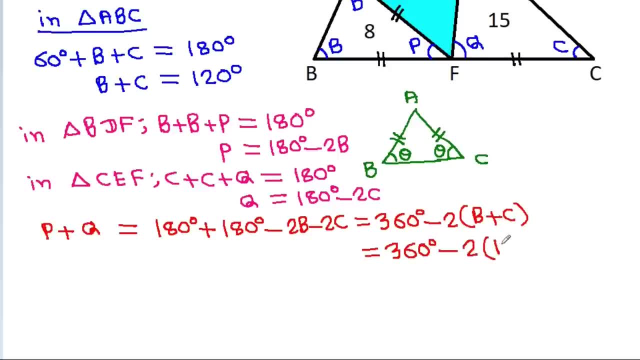 And it is 360 degree minus 2 times B plus C is 120 degree And it is 360 degree minus 240 degree And it is 360 degree minus 240 degree, that will be equal to 120 degree. 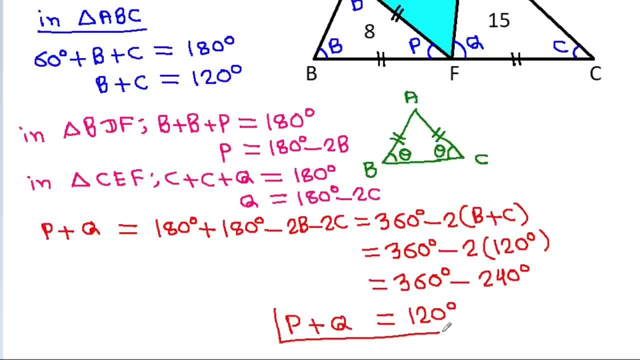 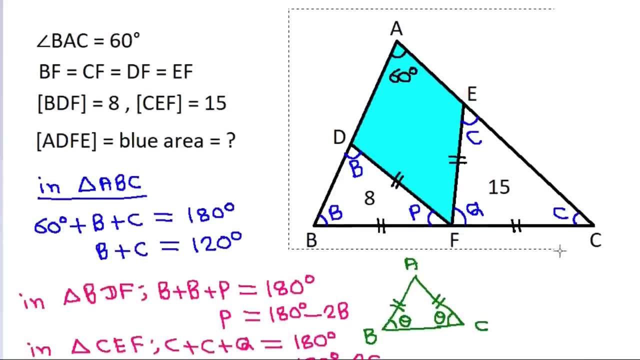 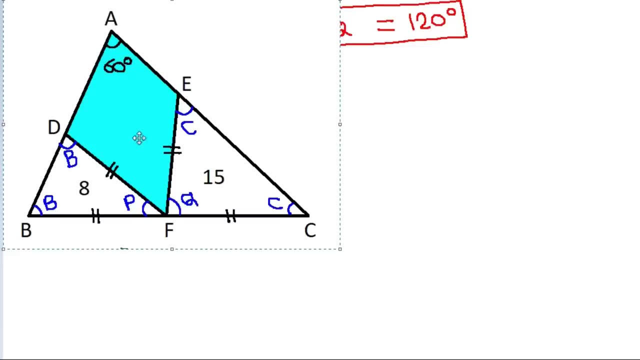 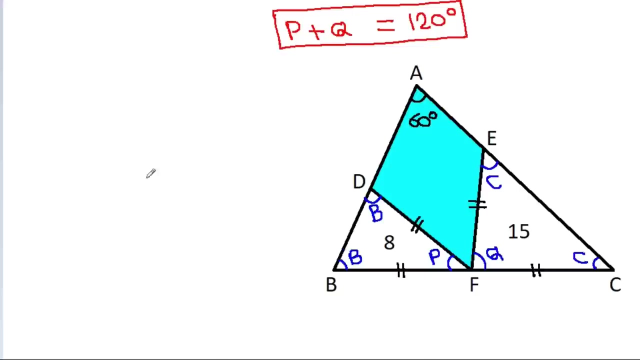 So P plus Q, it is 120 degree. So P plus Q, it is 120 degree, and it will be equal to 122.. And now P plus angle, DFE plus Q, it will be equal to 180 degree. 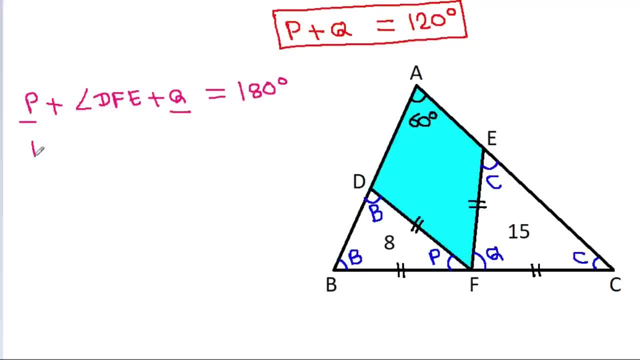 And P plus Q is 120 degree, Plus angle DFE it is 180 degree. So angle DFE it will be equal to 60 degree. So this angle it is 60 degree And if we join DE, then inter-angle DEF it is DEF, DF it is equal to EF. 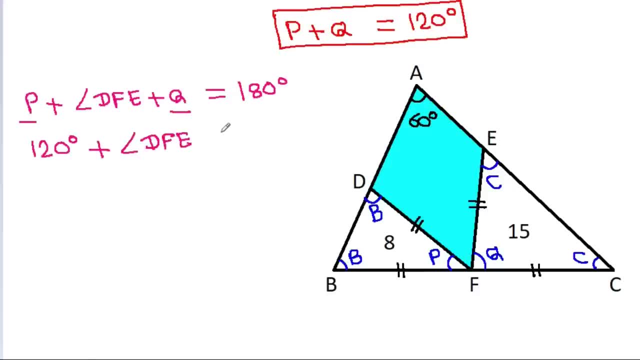 Plus angle df e, it is 180 degree. So angle df e it will be equal to 60 degree. So this angle, it is 60 degree. And if we join d enfin, d e, then in triangle d e, f, it is d e, f, d f, it is equal to e f and this angle is 60 degree. 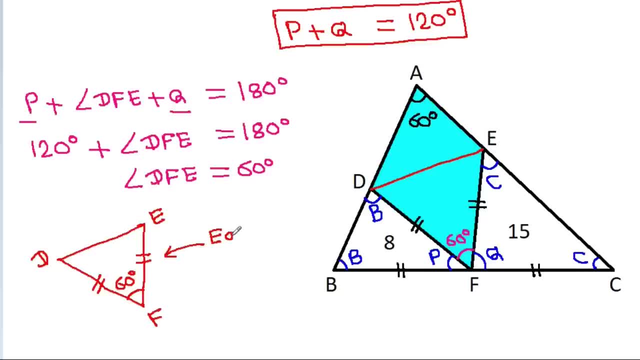 60 degree. that means it will be equilateral triangle. so these two angles will be 60 degree and DE it will be equal to DF, that will be equal to EF, and these angles are 60 degree. and now this angle: it will be 180 degree minus 60 degree. that means it will be equilateral. 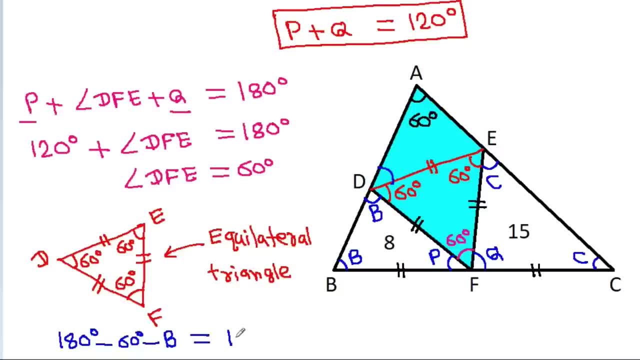 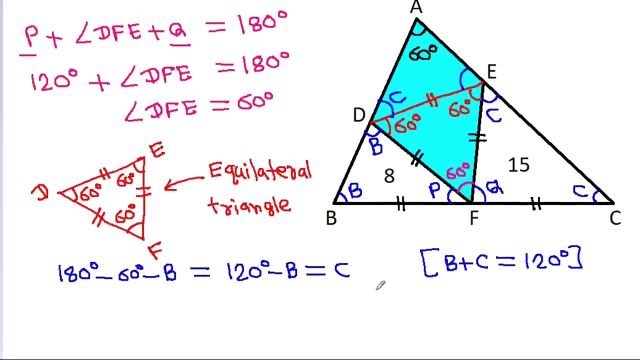 degree minus B, that is equal to 120 degree minus B, and it will be equal to C, because B plus C it is equal to 120 degree. so this angle is C and this angle it will be 180 degree minus 60 degree. 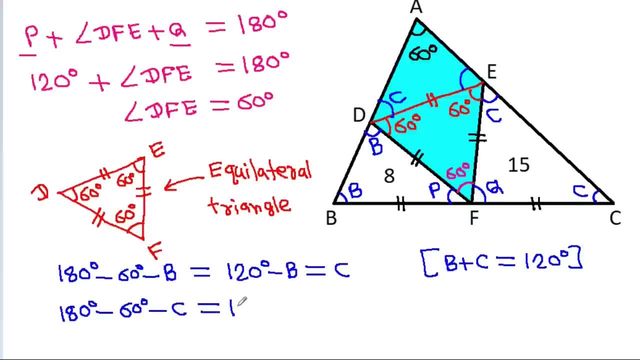 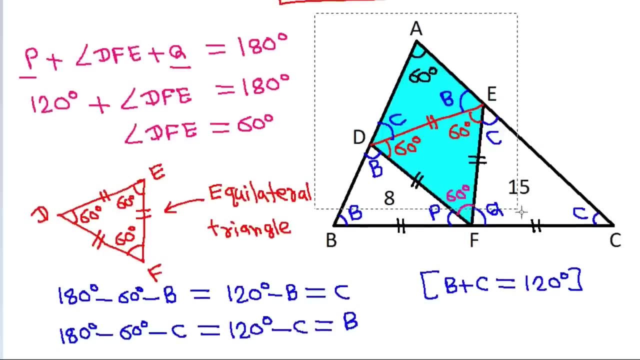 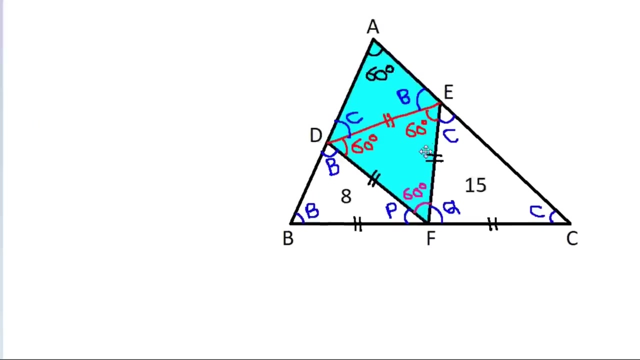 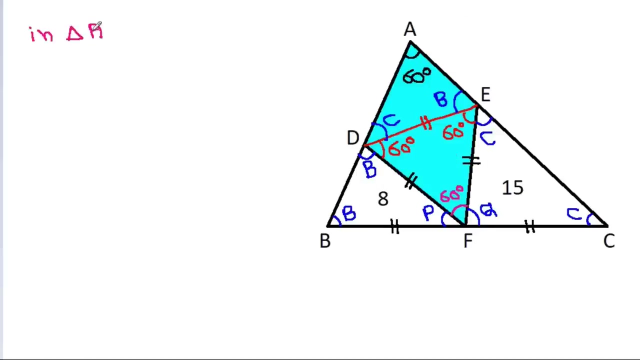 That will be equal to 120 degree minus C and it will be B. so it is B. and now we will use angle A B C and angle A E D in triangle A B C and triangle A E D. 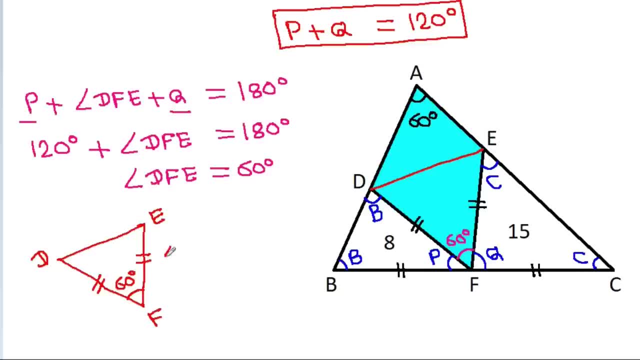 And this angle is 60 degree. That means it will be equivalent. So these two angles will be 60 degree And DE it will be equal to DF, that will be equal to EF, And these angles are 60 degree. 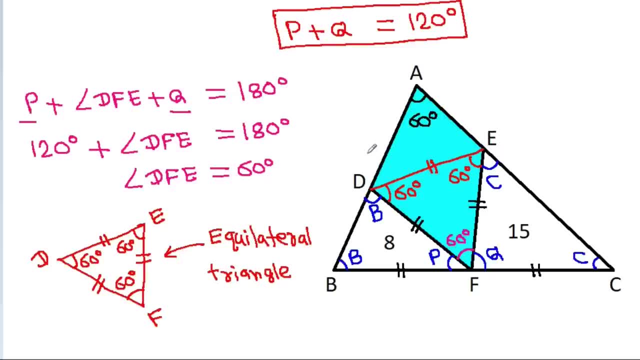 And now this angle: it will be 180 degree minus 60 degree minus B, that is equal to 120 degree minus B, And it will be equal to C, Because B plus C it is equal to 100.. 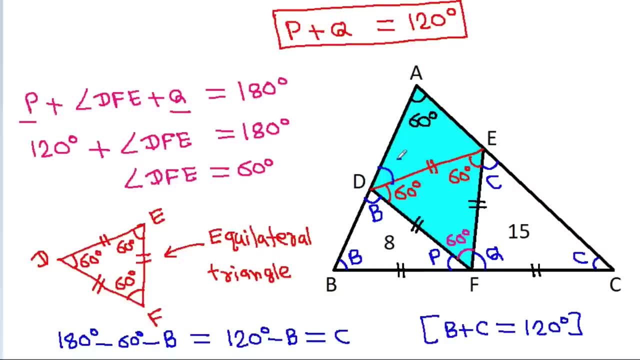 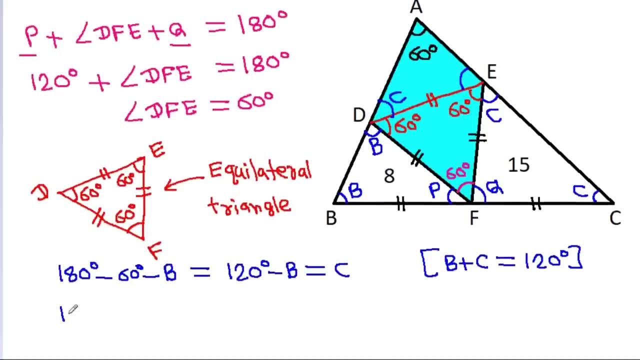 So now, which angle? That will be equal to B. Now, this angle is 50 degree. The angle is proportional to the angle at which it is a length of 2D in the calf. Alright, So this angle is C. 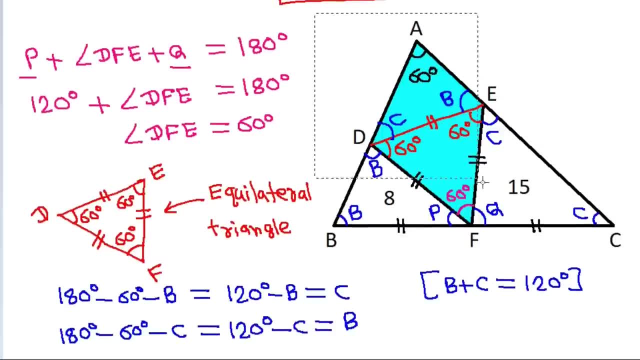 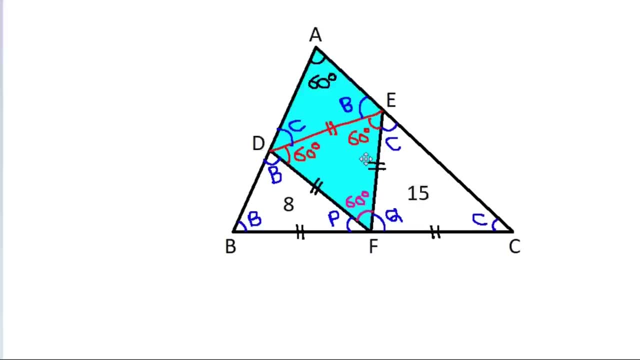 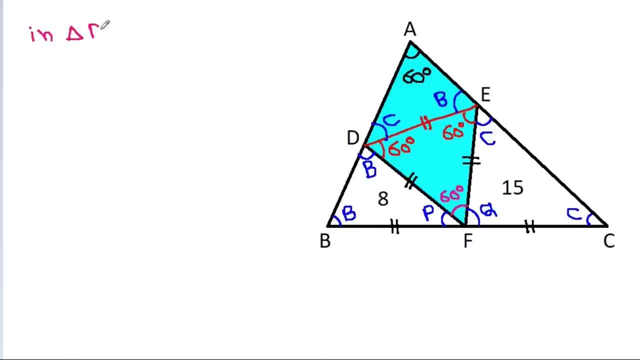 Now in triangle A, B, C and triangle A E D. angle A B C it is equal to angle A, E, D and angle A C- B, it is equal to angle A, D, E. 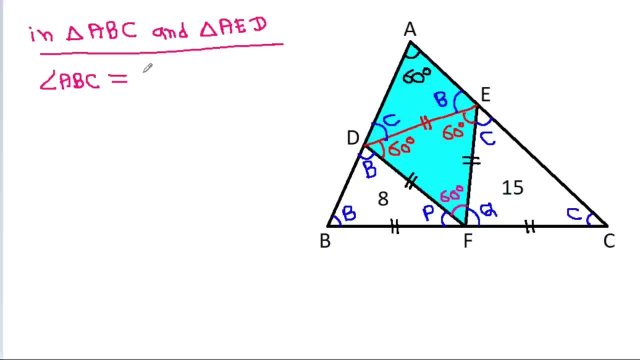 angle A, B, C it is equal to angle AE, D and angle ACB it is equal to angle ADE and angle ACB it is equal to angle ADE. So, by angle angle similarity, triangle ABC it will be similar to triangle AED. 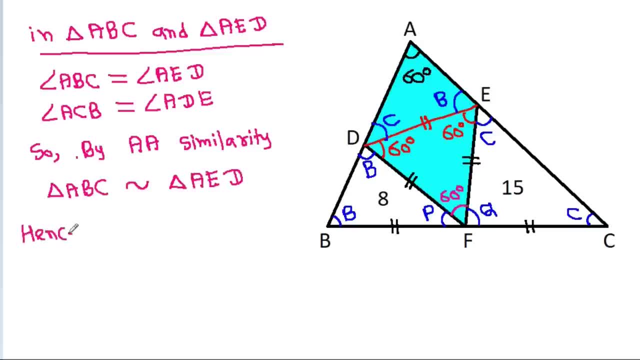 Hence, area of ABC by area of AED, it will be equal to BC squared by ED squared. And suppose ED is X, Then this will be X, this will be X and this will be X. this will be X. 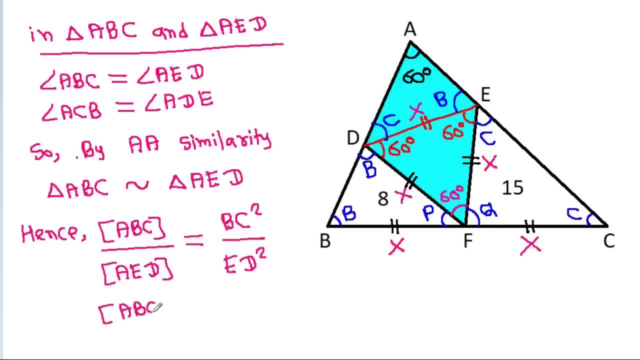 So area of ABC by area of AED, it is equal to BC. it is X plus X squared by ED is X squared, Okay, And it is 2X squared by X squared. that is equal to 4X squared by X squared and it will be equal to 4.. 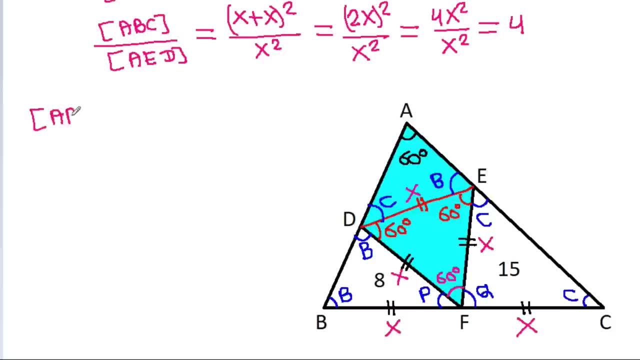 So area of AC- ABC- it will be equal to 4 times area of AED and area of BCED it will be equal to area of ABC minus area of AED and it is 4 times area of AED minus area of AED. that will be: 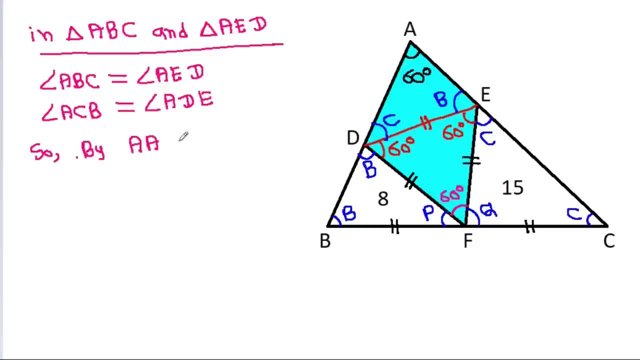 So by angle, angle, similarity, similarity, triangle A B C, it will be similar to triangle A E D, Hence area of A B C. by area of A E D, it will be equal to B C squared. 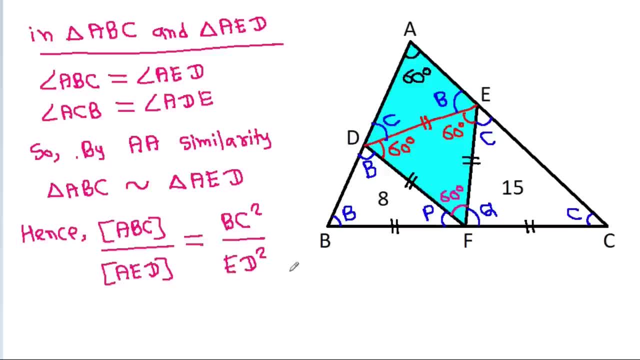 by E, D squared, And suppose E D is x, then this will be x, this will be x and this will be x, this will be x. So, area of A, B, C by area of A E D. 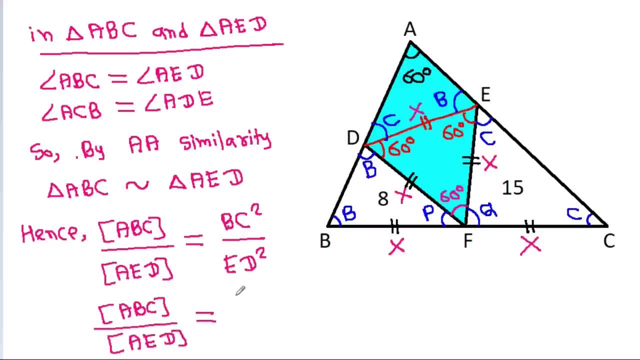 it is equal to B C squared, It is equal to B C squared, It is equal to B C squared, It is equal to B C. it is x plus x squared by E. D is x squared, and it is 2x squared by x squared. 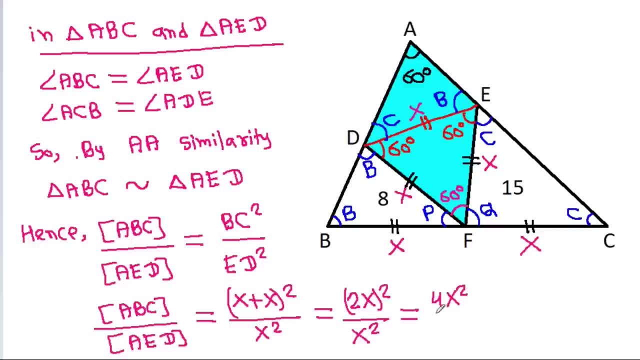 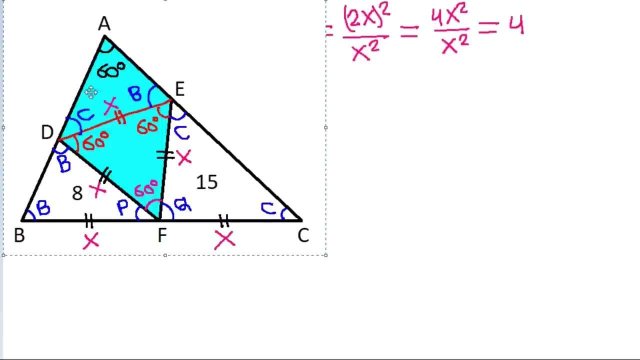 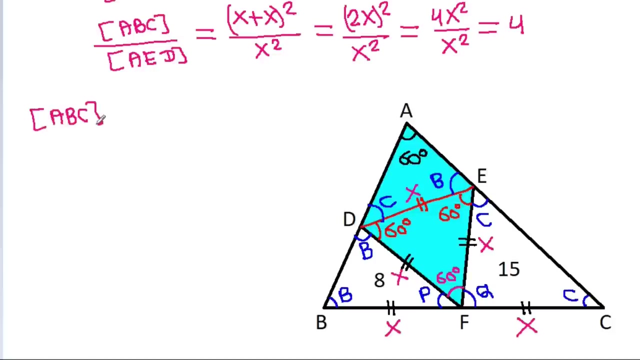 that is equal to 4x squared by x squared, and it will be equal to 4.. So area of A, B, C: it will be equal to 4x. area of A, E, D and area of B. 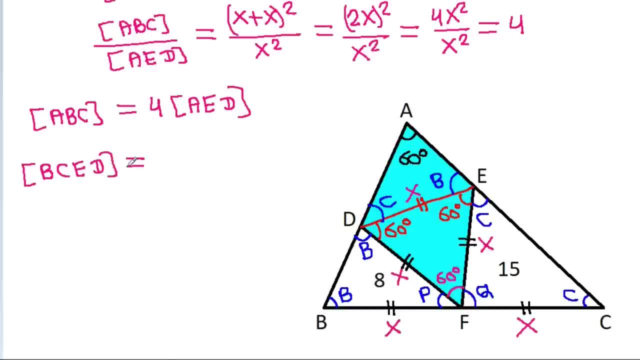 CED, it will be equal to area of ABC minus area of AED and it is 4 times area of AED minus area of AED. that will be equal to 3 times area of AED. it is area of BCED. 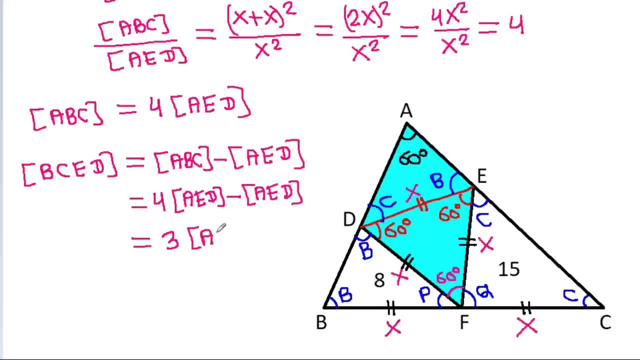 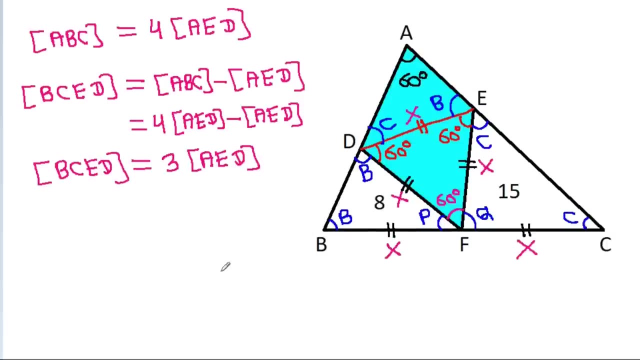 equal to 3 times area of AED. It is area of BCED And now area of CEF. by area of BDF it will be equal to area of CEF is 15 times area of CEF. by area of BDF is 8.. 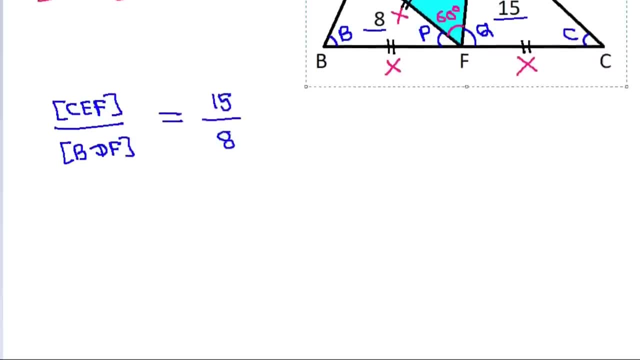 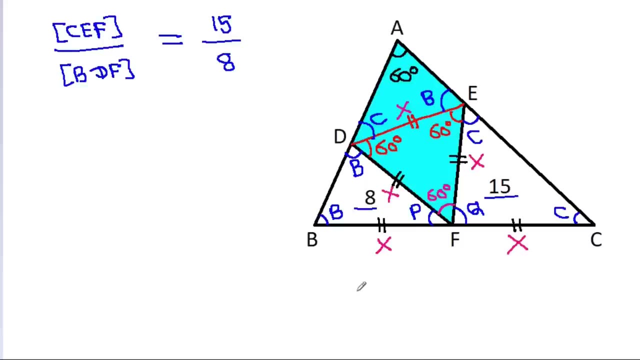 And in any triangle ABC it will be equal to area of CEF. Okay, Okay, Okay. So if BC is A and AC is B and this angle is theta, then area of ABC it is equal to 1 by 2 times A times B times, sine theta. 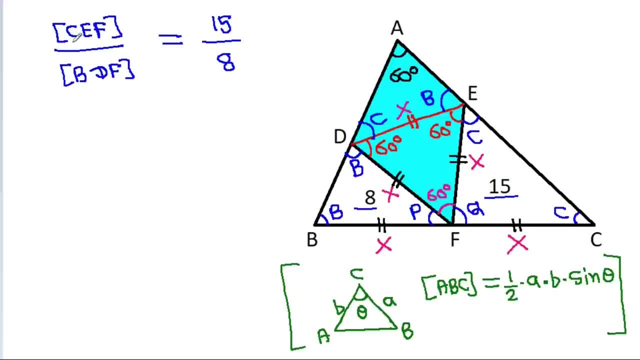 So area of CEF: Okay, Okay, It will be 1 by 2 times CF times EF times sine Q. by area of BDF, It will be 1 by 2 times BF times DF times sine P. It is equal to area of ADF plus BDF. 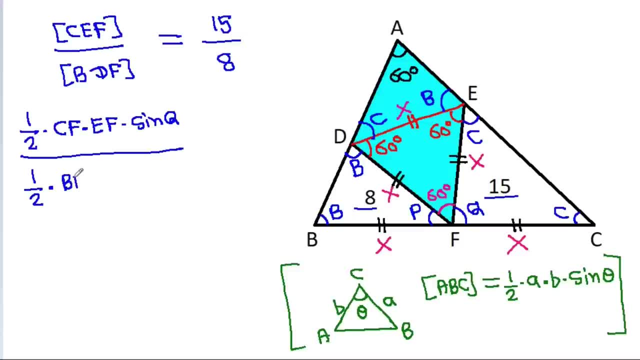 Okay, Okay, Okay, Okay. So it will be equal to 3 times BDF minus area of AED, minus area of BDF, And it will be equal to 3 times area of BDF. Okay, Okay, Okay. 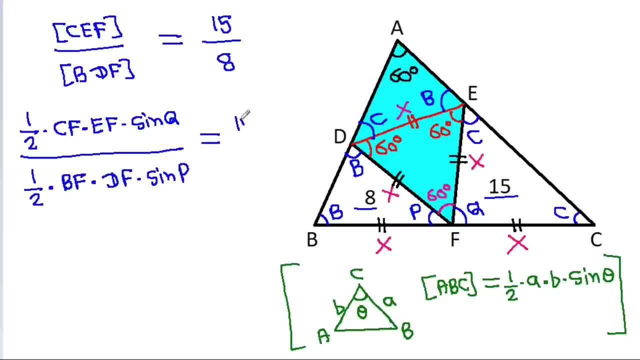 Okay, Okay, Okay Okay, 15 by 8 and 1 by 2 will get cancelled, and cf is x times ef is x times sine and we have: p plus q is equal to 120 degree. so q will be equal to 120 degree minus p by bf is x. 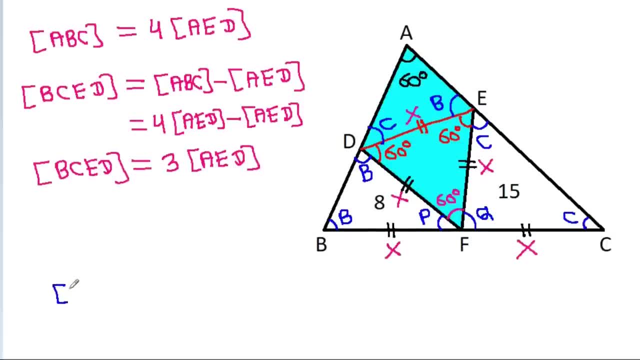 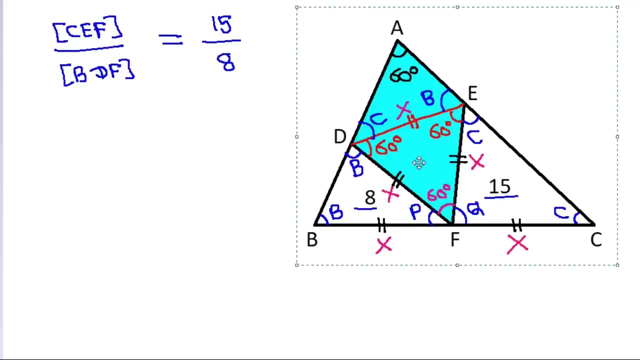 And now area of CED: CEF by area of BDF it will be equal to: area of CEF is 15. by area of BDF is 8.. And, and, and GOD, in any triangle, in any triangle, in any triangle, ABC, If BC is A and AC is B and this angle is theta, then research of ABC. 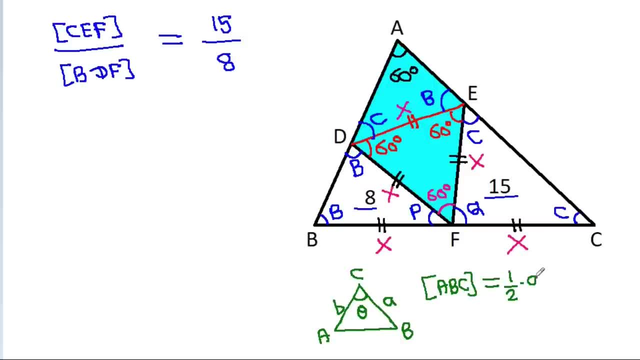 It is equal to function of AN Д and A B. It is equal to function of AN DC and weight of dub Y trashedine B. Poor English woman. error in English. error in English: 1 by 2, times A times B, times sin theta. so area of CEF it will be 1 by 2, times CF. 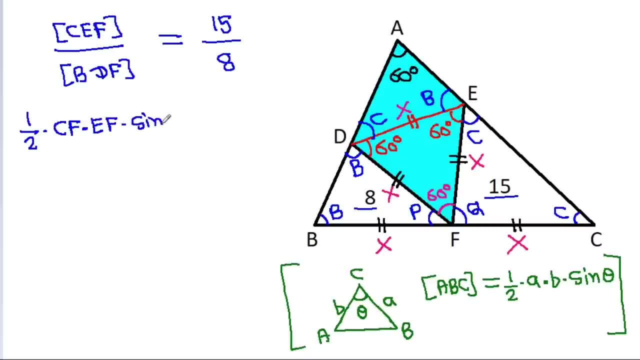 times EF times sin Q, by area of BDF, it will be 1 by 2, times BF times DF times sin P, it is equal to 15 by 8, and 1 by 2 will get. 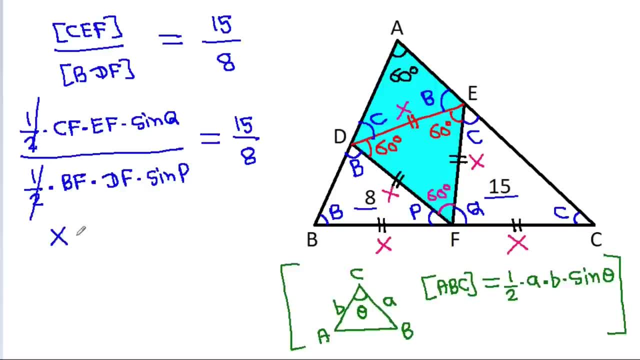 and CF is X times EF, is X times sin and we have: P plus Q is equal to 120 degree. so Q will be equal to 120 degree minus P by. BF is X times DF is X times sin P, it is equal to 15 by 8, and X will get constant. 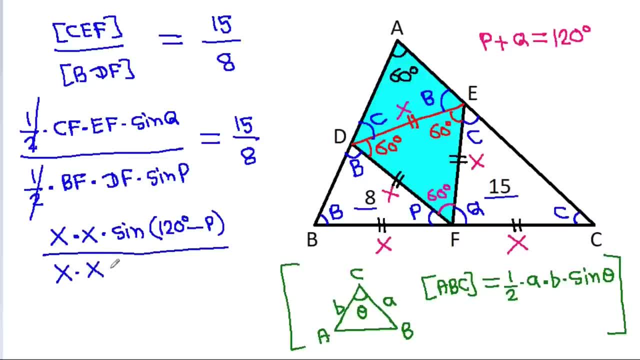 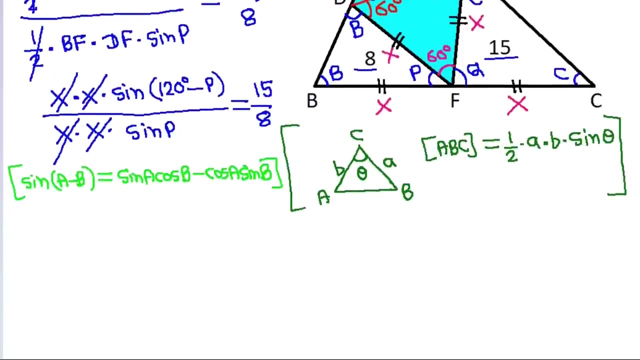 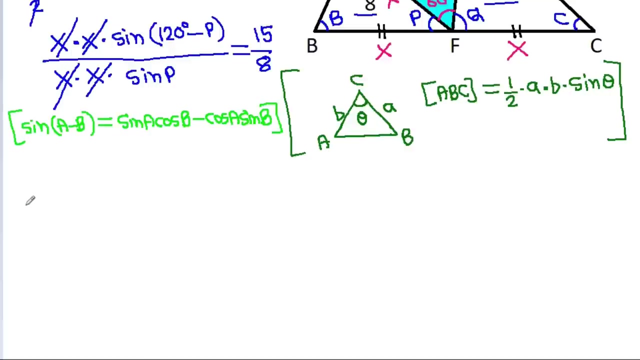 times df is x times sine p, it is equal to 15 by 8 and x will get cancelled. and again x will get cancelled and sine a minus b it is equal to sine a cos b minus cos a sine b. so sine 120 degree minus p, it will be sine 120 degree cos p minus cos 120 degree sine p. 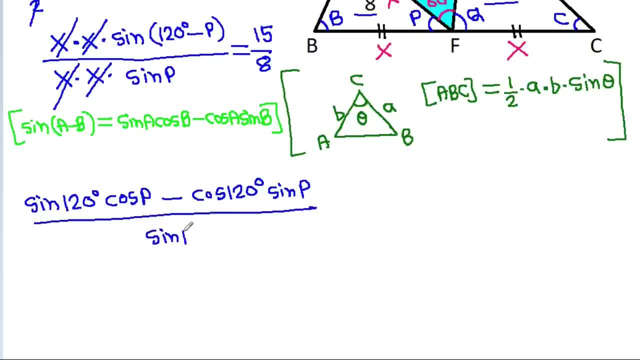 by sine p, it is equal to 15. by 8 and sine 120 degree, it is a square root of 3 by 2 times cos p. by sine p minus and cos 120 degree, it is minus 1 by 2 times sine p. by sine p, it is equal to 15 by. 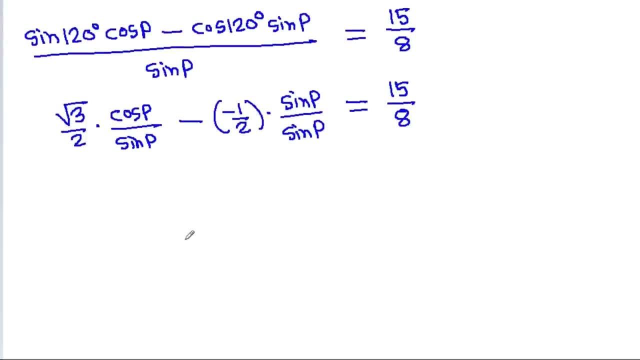 8 and it is a square root of 3 by 2 and sine p by cos, p will be tan p and here sine p will get cancelled, and it is plus 1 by 2. that is equal to 15 by 8, so a square root of 3. 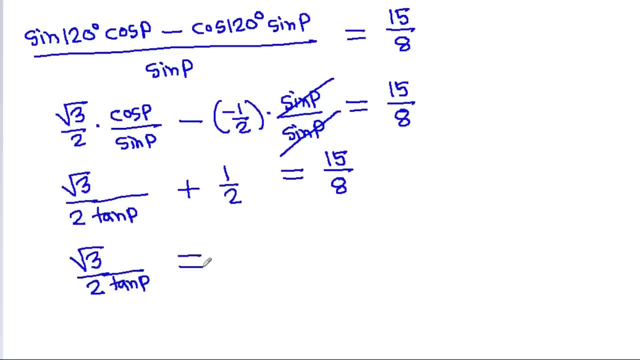 by 2 times tan p, it will be equal to 15 by 8 minus 1 by 2, that is, 15 by 8 minus 4 by 8, and it will be 11 by 8.. So tan p, it will be equal to a square root of 3 times 8 by 2 times 11 and 2 times 4. 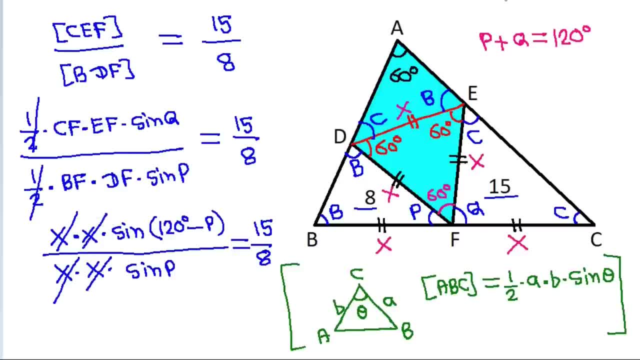 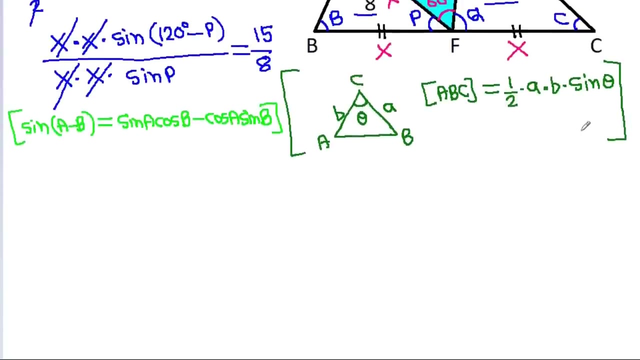 and again X will get constant and sin A minus B it is equal to sin A cos B minus cos A sin B. so sin 120 degree minus P it will be sin 120 degree cos P minus cos 120 degree. 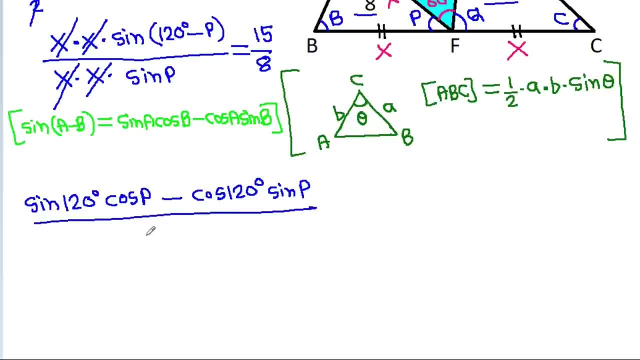 sin P. by sin P, it is equal to 15 by 8, and sin 120 degree it is a square root of 3, by 2, times cos P, by sin P minus and cos 120 degree. 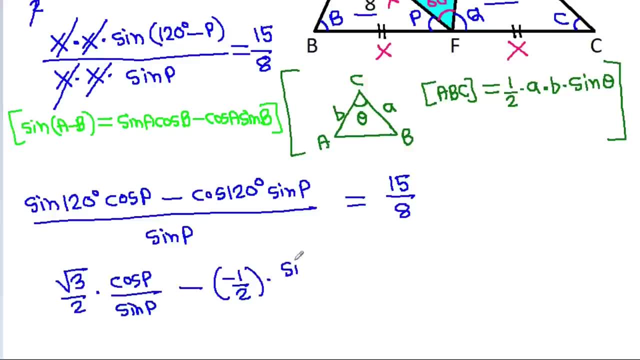 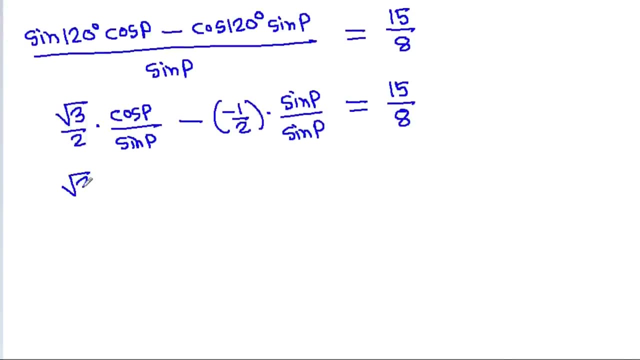 it is minus 1 by 2, times sin P. by sin P, It is equal to 15 by 8, and it is a square root of 3, by 2, and sin P by cos P will be tan P. 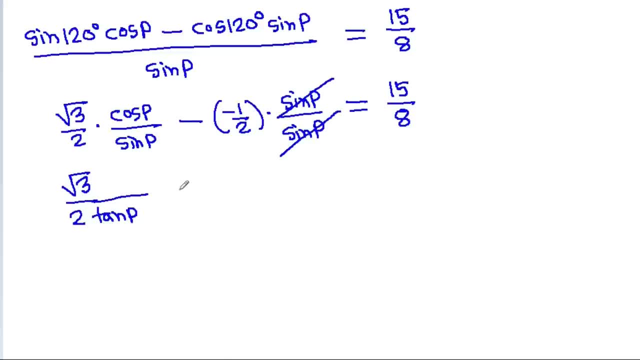 and here son P will get canceled, and it is plus 1 by 2. that is equal to 15 by 8.. So a square root of 3 by 2 times tan p, it will be equal to 15 by 8 minus 1 by 2, that is 15 by 8 minus 4 by 8, and it will be. 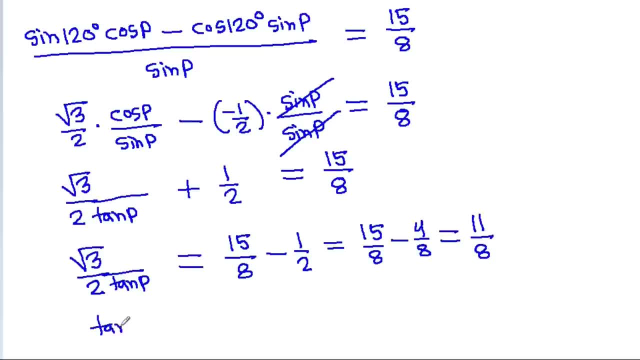 11 by 8.. So, tan p, it will be equal to a square root of 3 times 8 by 2 times 11, and 2 times 4 is 8.. So it is 4 times a square root of 3 by 11.. 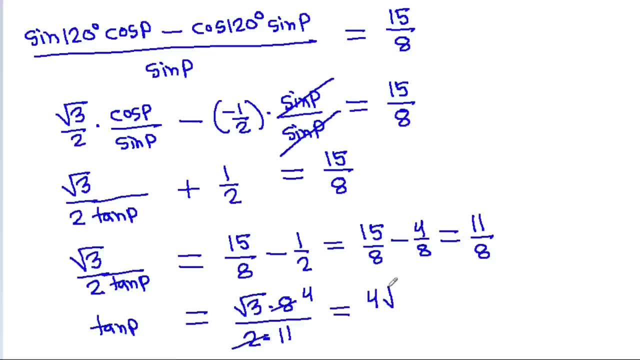 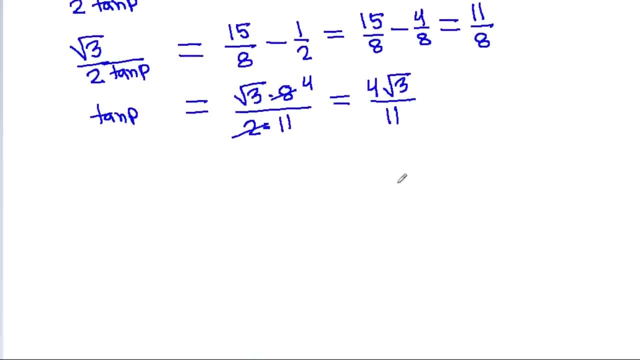 is 8, so it is 4 times a square root of 3 by 11.. and any triangle, this angle is 90 degree and this is perpendicular. this is base and this is hypotenuse. If this angle is theta, then tan theta it is equal to p by b and sine theta it is equal to p by h. 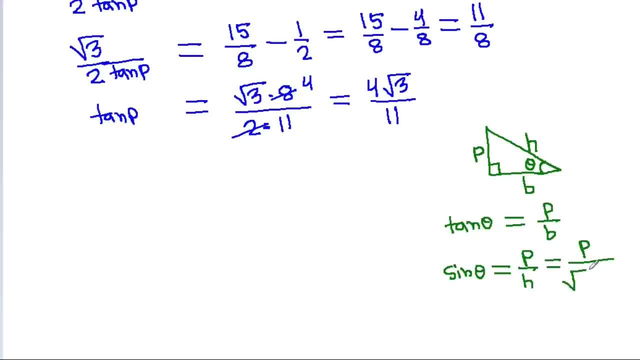 and it is p by h. spoiler to Chuckle: h is a square root of p square minus b square. and here we have tan. p is equal to 4 times a square root of 3 by 11.. so, sine p, it will be equal to 4 times a square root of 3. 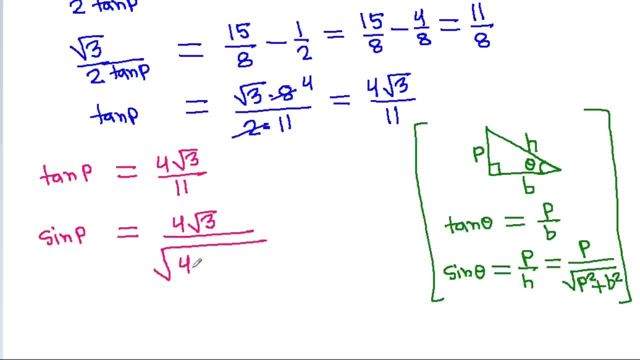 by a square root of 4 times a square root of 3: a square plus 11 a square, and it is 4 times a square root of 3 by a square root, and it is 48 plus 121, and it is 4 times a square root of 3. by a square root of 169, that is equal to 4. 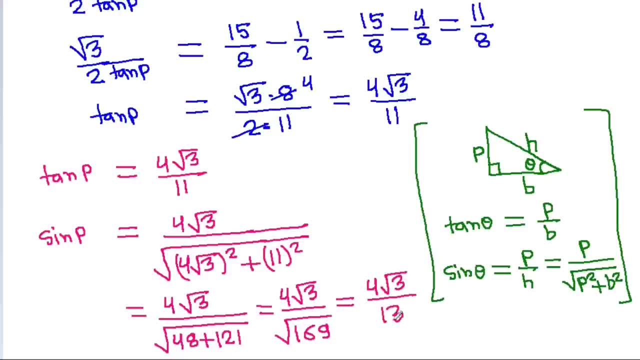 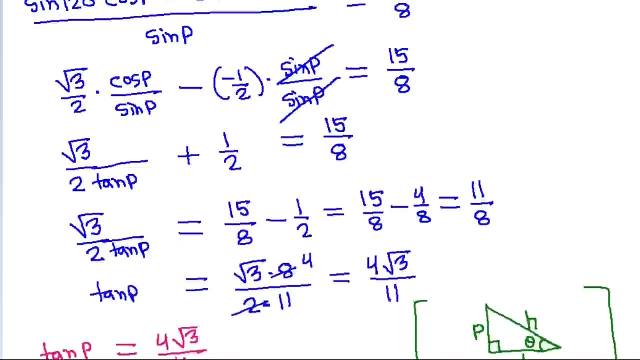 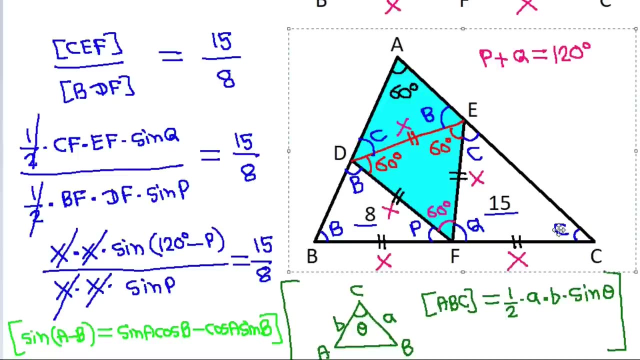 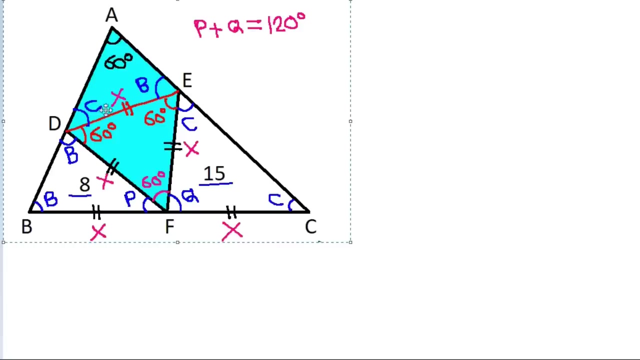 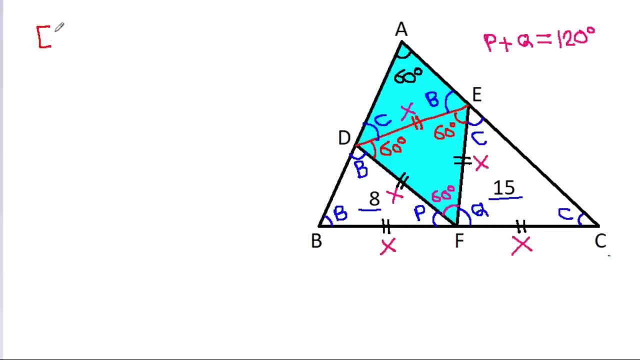 times a square root of 3 by 13, it is sin P. and it is 4 times a square root of 3 by 13, it is sin P. and We have: area of BDF is equal to 8 and area of BDF it is 1 by 2 times x times, x times. 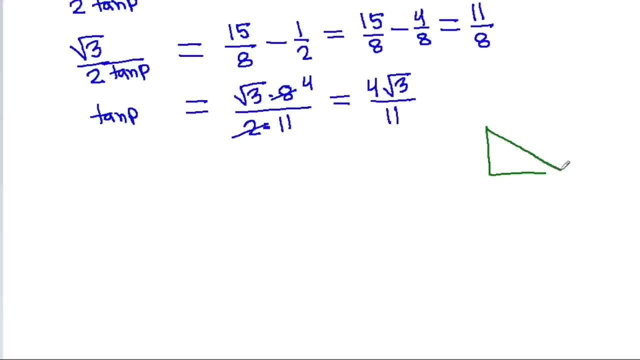 And in any triangle this angle is 90 degree and this is perpendicular, this is base and this is hypotenuse. If this angle is theta, then tan theta it is equal to p by b and sine theta it is equal to p by h. 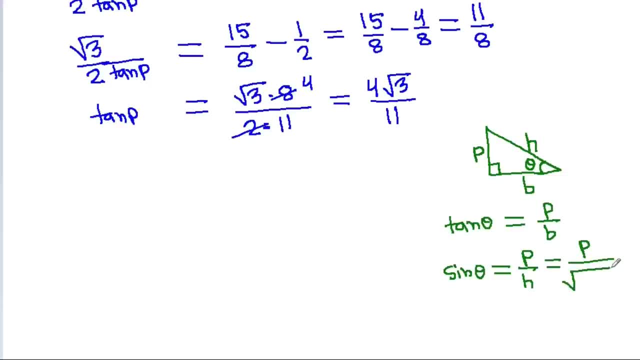 And it is. p by h is a square root of p square plus b square, And here we have tan. p is equal to 4 times a square root of 3 by 11.. So, sine p, it will be equal to 4 times a square root of 3. 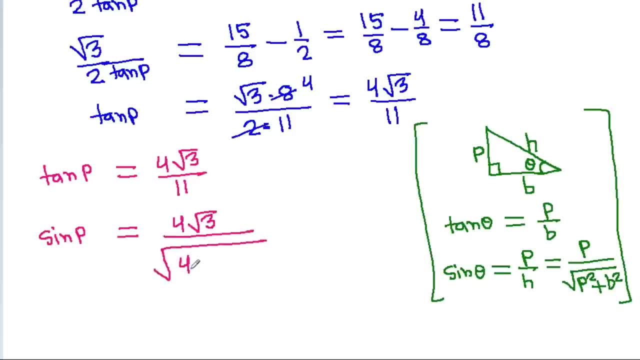 by a square root of 4 times a square root of 3: a square plus 11 a square, and it is 4 times a square root of 3 by a square root, and it is 48 plus 121, and it is 4 times a square root of 3. by a square root of 169, that is equal to 4. 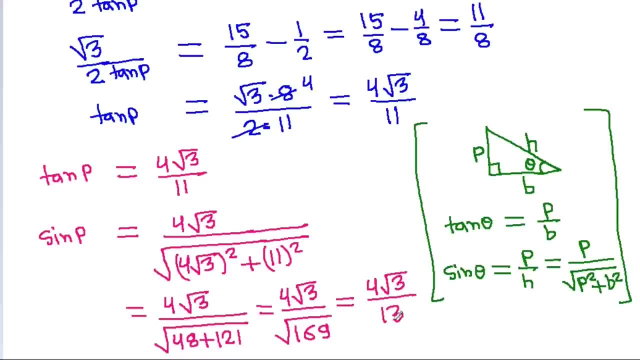 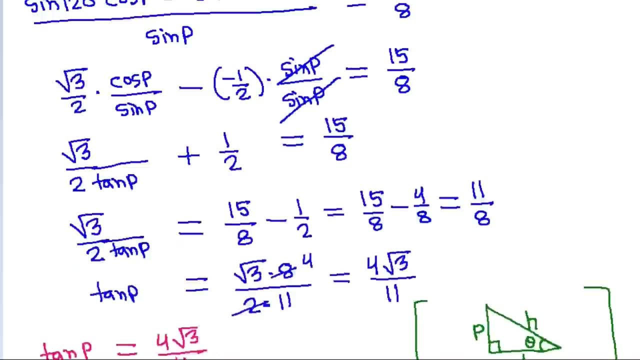 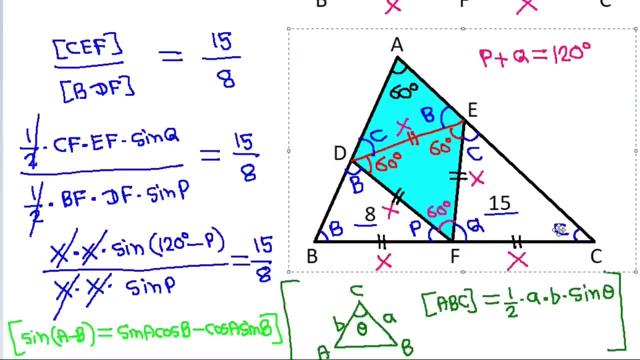 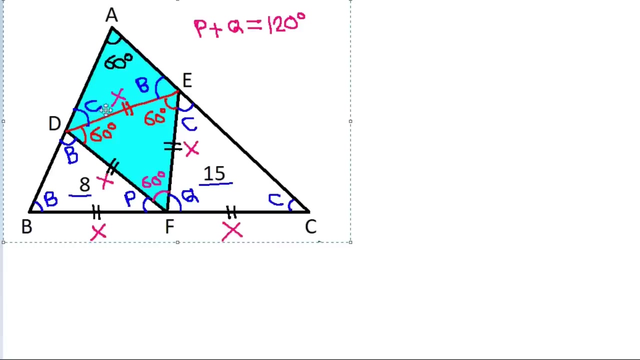 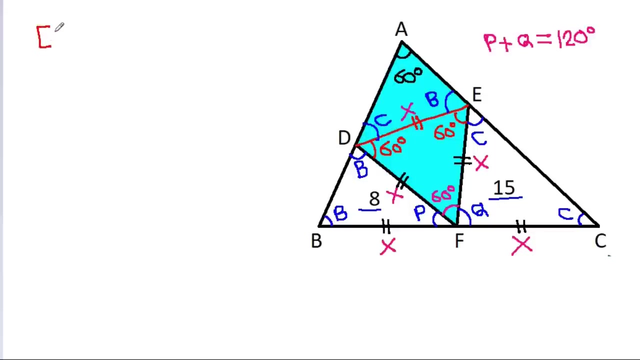 times a square root of 3 by 13, it is sin P. and it is 4 times a square root of 3 by 13, it is sin P. and we have: area of BDF is equal to 8 and area of BDF it is 1 by 2 times x times x. 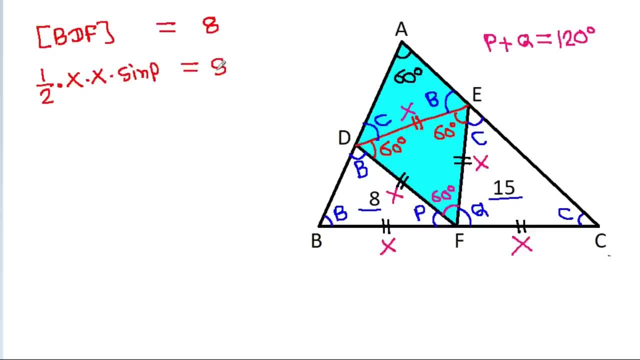 times sin P, that is 8, and it is 1 by 2 times x times x times and sin P, it is 4 times a square root of 3 by 13, that is equal to 8, and 2 times 2 is 4, so x a. 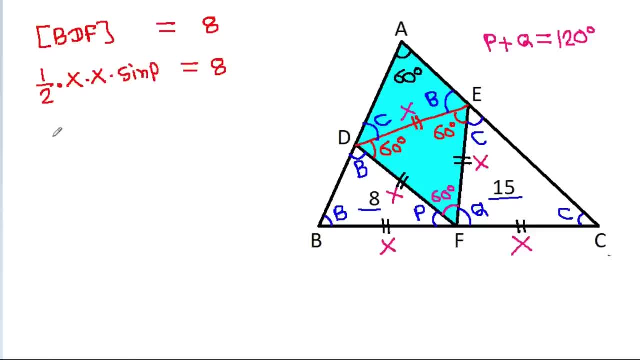 sin, that is 8 and it is 1 by 2 times, x times x times and sin it is 4 times s square root of 3 by 13,. that is equal to 8, and 2 times 2 is 4, so x square it will. 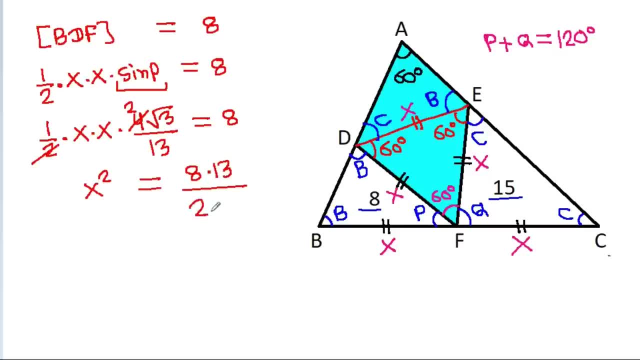 be equal to 8 times 12.. 13 by 2 times a square root of 3.. So x square, it is equal to 2 times 4 is 8 and 13 times 4 is 52 by a square root of 3.. 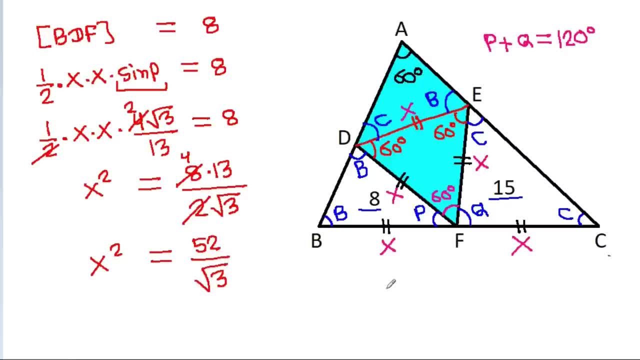 And in any equilateral triangle, a b c, if a, b is equal to a, c is equal to b c. that is a then area of a b c. it is equal to a square root of 3 by 4 times a square. 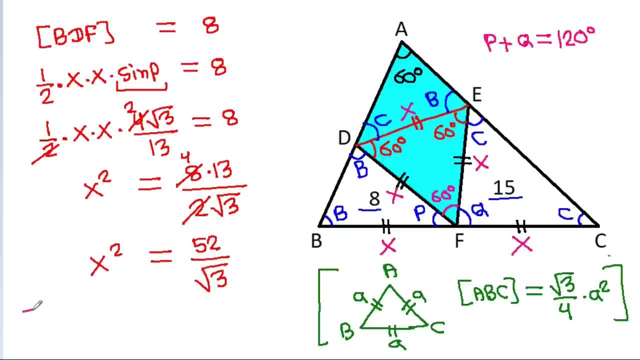 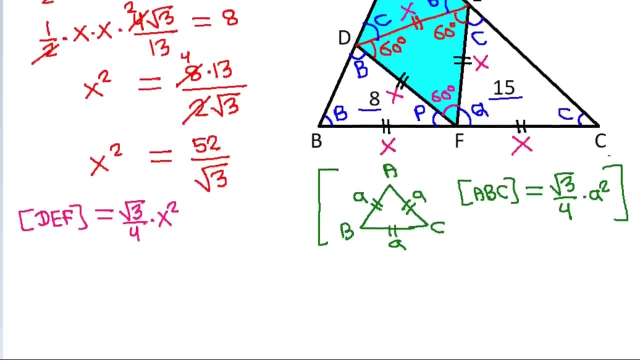 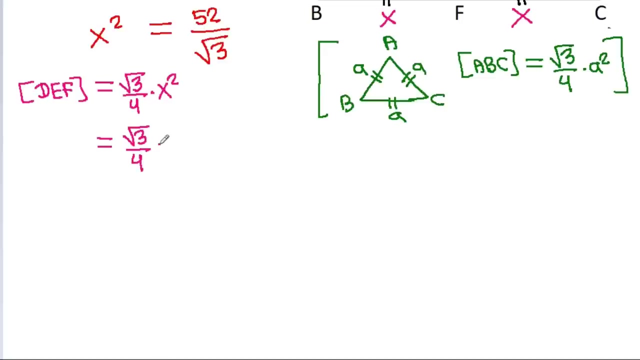 So area of d e f. it will be equal to a square root of 3 by 4 times x square And it is a square root of 3 by 4 times and x square is 52.. By a square root of 3 and a square root of 3 will get constant and 4 times 13 is 52.. 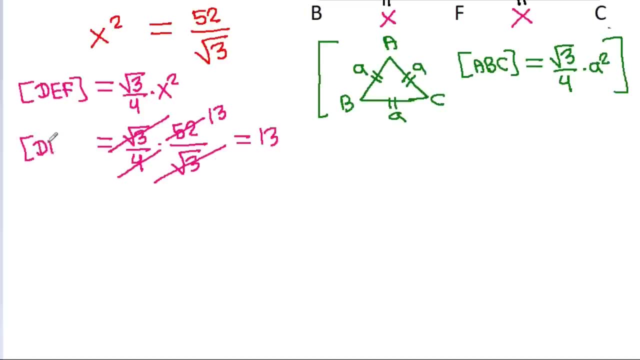 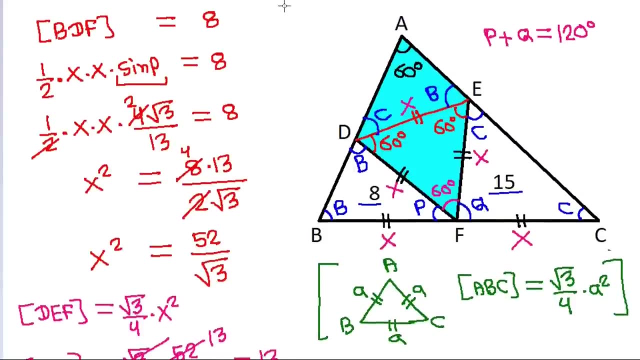 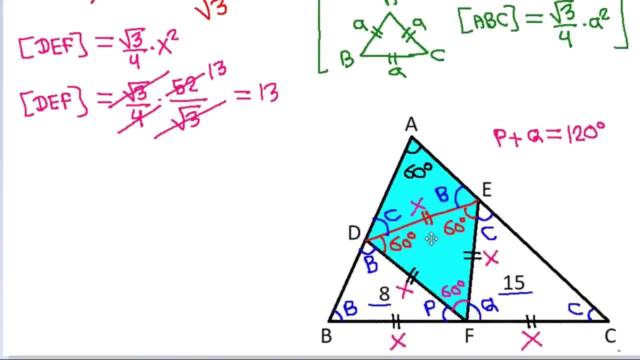 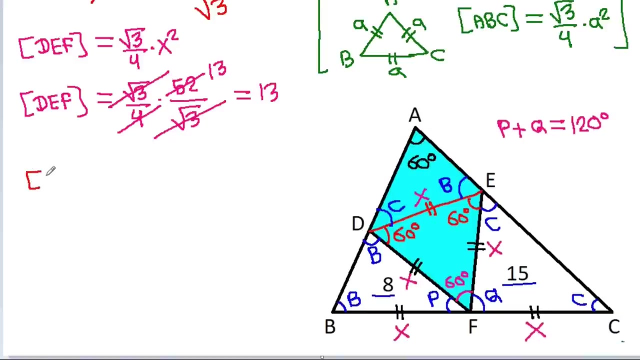 So it is 13.. Area of d e, f is 13 and we have area of b, c, e, d is equal to three times area of a e d And this area is 13.. So area of b, c, e d: it will be 8,. 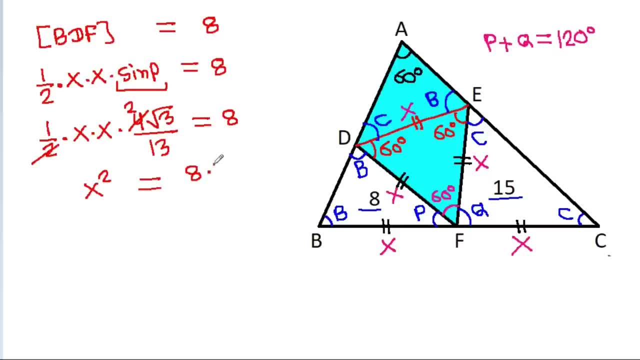 square it will be equal to 8 times 13 by 2 times a square root of 3. so x a square it is equal to: 2 times 4 is 8 and 13 times 4 is 52 by a square root of 3 and in any equilateral. 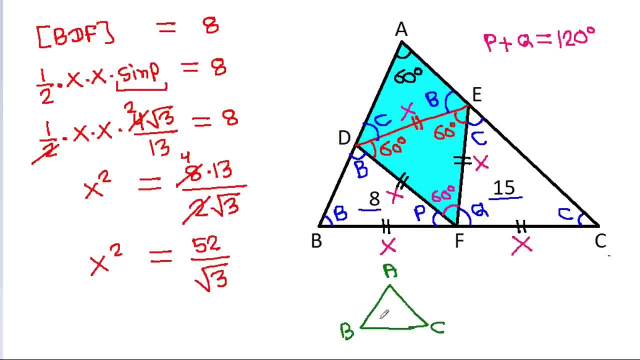 trend, in any equilateral trend, in any equilateral trend. angle a, B, C if AB is equal to AC is equal. angle a B- C if AB is equal to AC, is equal. angle a, B- C if AB is equal to AC, is equal to BC. that is a, then area of ABC. it is. 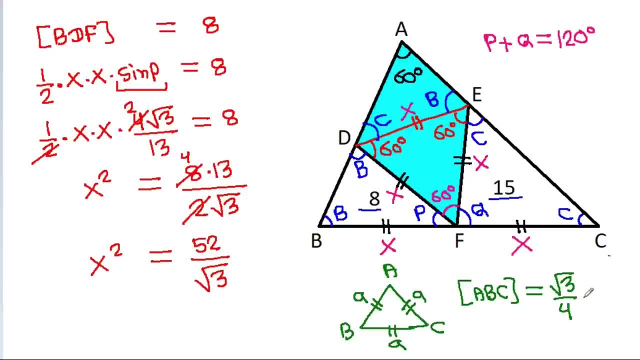 to BC. that is a then area of ABC. it is to BC that is a then area of ABC. it is equal to a square root of 3 by 4 times a, equal to a square root of 3 by 4 times a, equal to a square root of 3 by 4 times a square. so area of D. 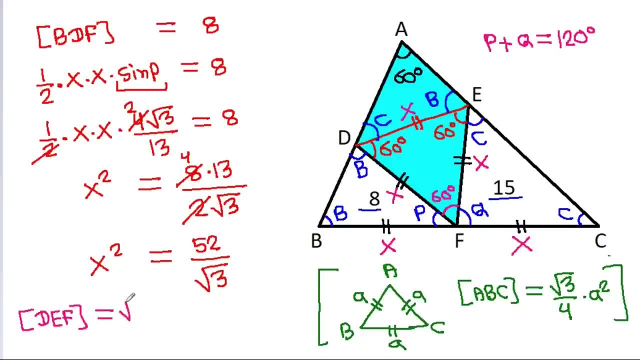 square, so area of D square, so area of D EF. it will be equal to a square root of 3 EF. it will be equal to a square root of 3 EF. it will be equal to a square root of 3 by 4 times X: a square, and it is a square. 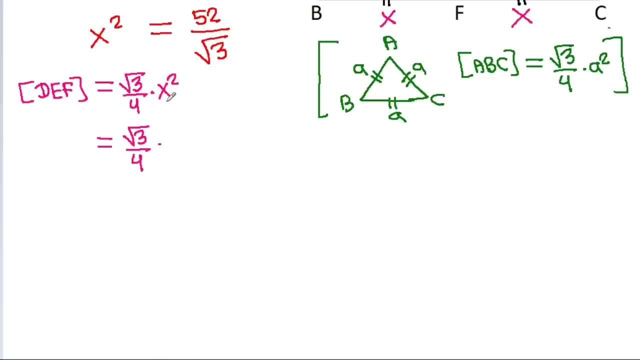 by 4 times, and X a square is 52 by a by 4 times and X a square is 52 by a by 4 times and X a square is 52 by a square root of 3 and a square root of 3. 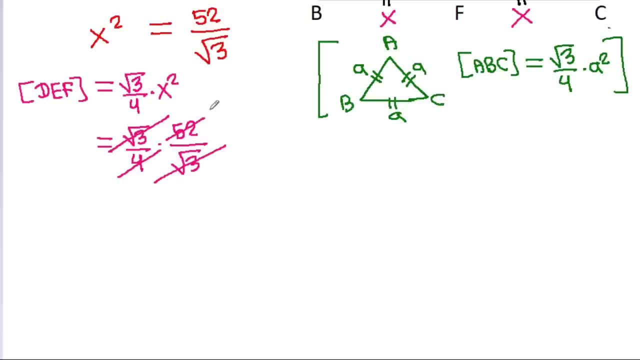 square root of 3 and a square root of 3, square root of 3 and a square root of 3, will get constant, will get constant, will get constant. and 4 times 13 is 52, so it is 13 area of, and 4 times 13 is 52, so it is 13 area of. 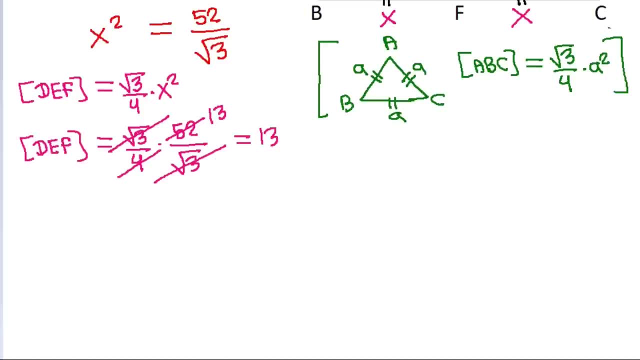 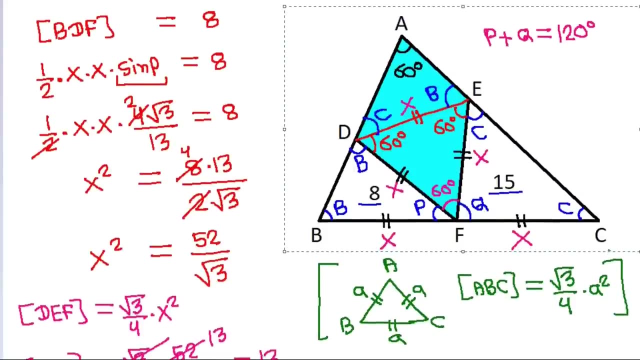 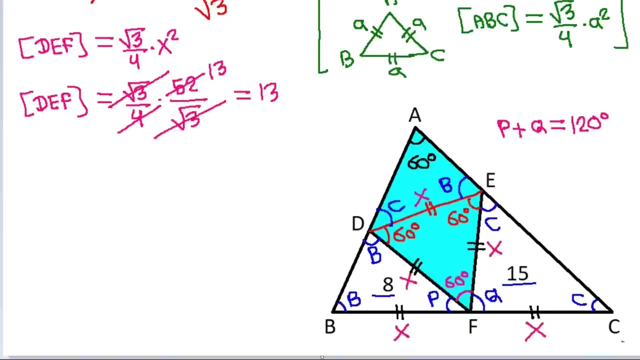